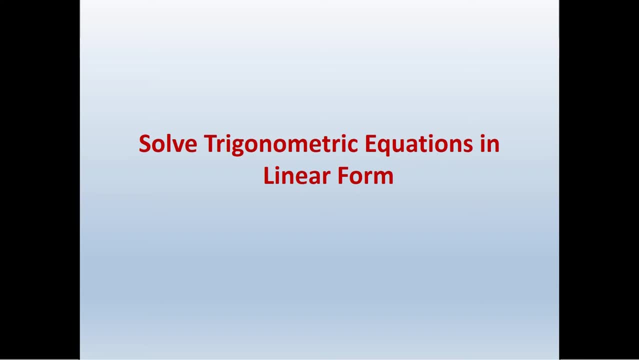 In this video we're looking at solving trigonometric equations in linear form. So how do we do that? Well, let's do an example real quick. We've got something as basic as this: Solve sine x equals square root of 3 over 2.. All right, so from the unit circle we know that there. 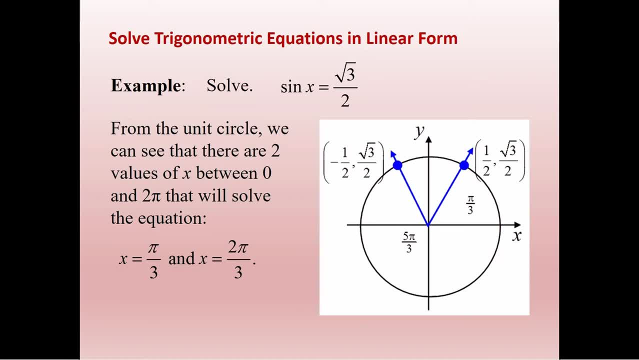 are two values of x between 0 and 2 pi. that'll solve this equation right, Where we know that if we're talking about sine, we're talking about the y value, So we're talking about the y value being square root of 3 over 2.. That happens here and here, So this is at pi over 3. 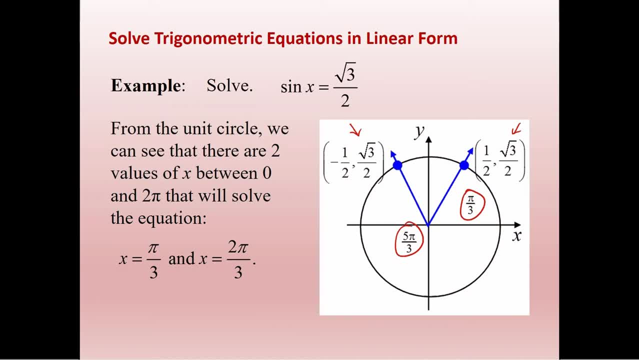 and at 5 pi over 3, okay. 5 pi over 3.. That's not 5 pi over 3.. That's 2 pi over 3, okay. So we know that that's where it happens, Those two values. So that means that. 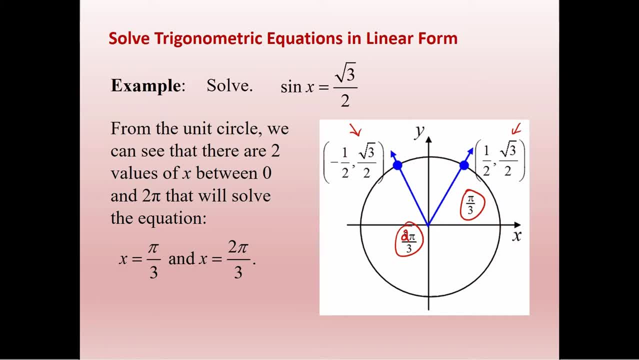 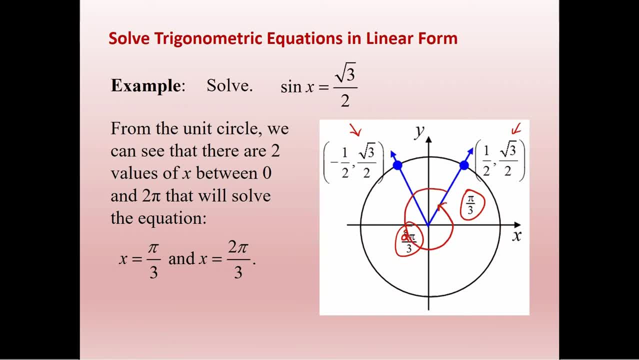 you're going to be able to solve this equation right If we think about this. you're going to be able to solve this equation right If we think about this pi over 3, but if we add 2 pi and get a coterminal angle, that will also work. Or if we subtract 2 pi. 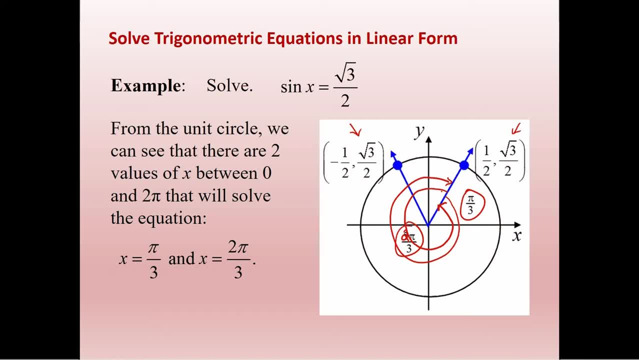 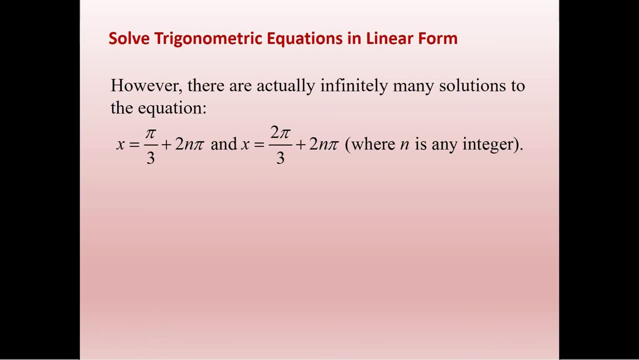 and get back this direction. we know that these are going to be terminal, coterminal angles and they're all going to have the same solution right. So we know that we can add. we say 2n pi, So we're adding n multiples of pi, where n is just some integer. So we add 2 pi. 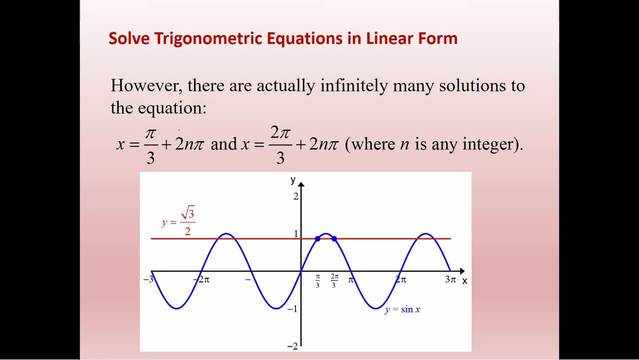 4 pi, 6 pi negative 2 pi, negative 4 pi, etc. It looks like this basically: So there's a line that will hit the square root of 3 over 2 infinitely many times for every adding 2 pi. 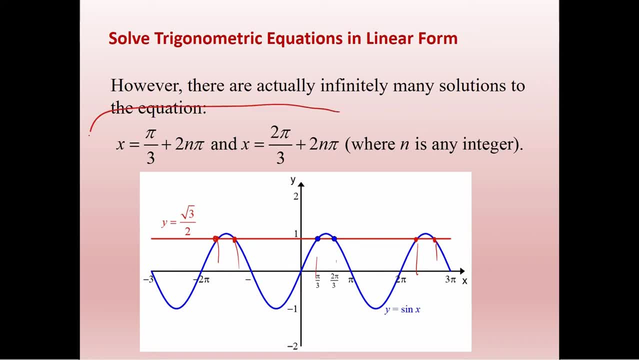 Every hump. okay, So this is our actual general solution. Anytime we're talking about sine or cosine, we're always going to add that plus 2n pi. But if we're talking about عة, well, sine cosine, cosecant and secant, all of those have a period of 2 pi. If we're talking 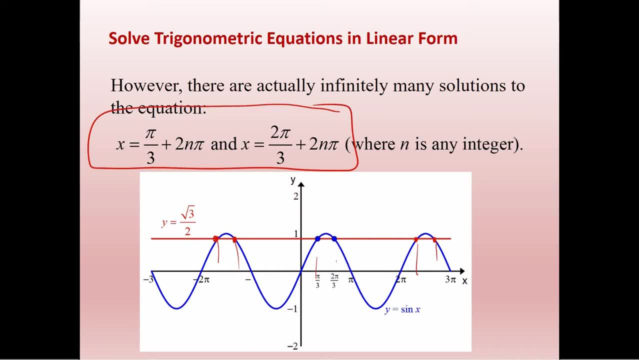 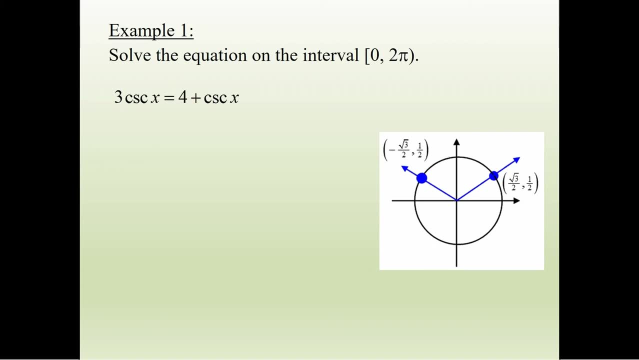 about tangent or cotangent, then we just say plus n, pi. okay. So let's do an actual example here: 3 cosecant x equals 4 plus cosecant x. So the first way that we learn how to solve equations like this is to isolate our variable or isolate our function. In this case, cosecant shows up. 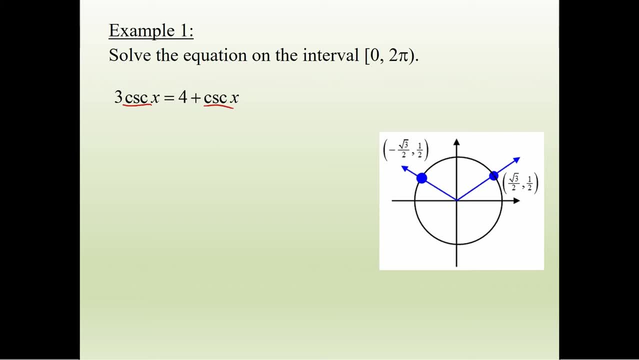 right. So if I can get cosecant by itself, then I can solve my equation. So I'm going to say: all right, so I have 3 cosecant. I'm going to subtract cosecant x. I get 3 minus 1 is 2, cosecant x equals 4.. We divide by 2. We get cosecant x equals 4 over 2. 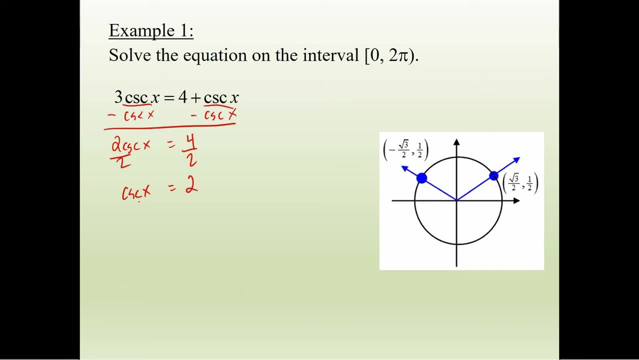 is just 2.. But this is cosecant and we don't really deal with cosecant. So we're going to say sine x equals 1, half right, Because cosecant is the reciprocal of sine and 2, the reciprocal is: 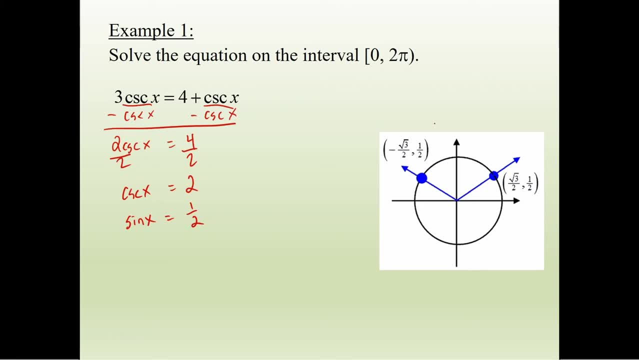 1 half. So we know that sine of 1 half occurs here and here. Where is this? Pi over 6 and 5 pi over 6.. So what does that mean? That means our solution on the interval from 0 to 2 pi. 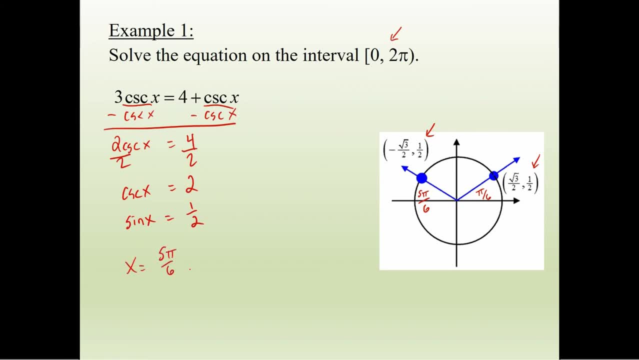 is just: x equals 5, pi over 6 and pi over 6.. These are the only two places on the unit circle, the interval from 0 to 2 pi. Now, if we didn't have that, if that weren't there, 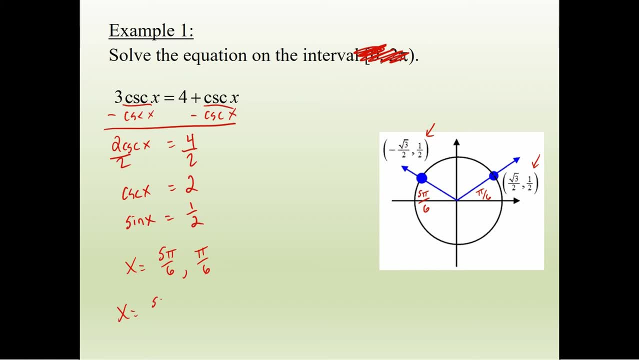 and we just wanted the general solution. then we would say that x equals 5 pi over 6 plus 2 n pi, and x equals pi over 6 plus 2 n pi, And that would be the general solution. okay, Which we'll.